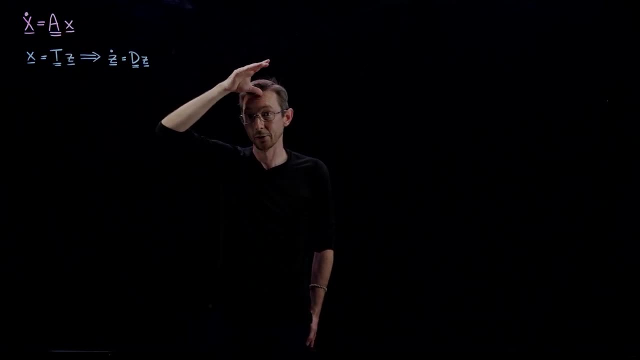 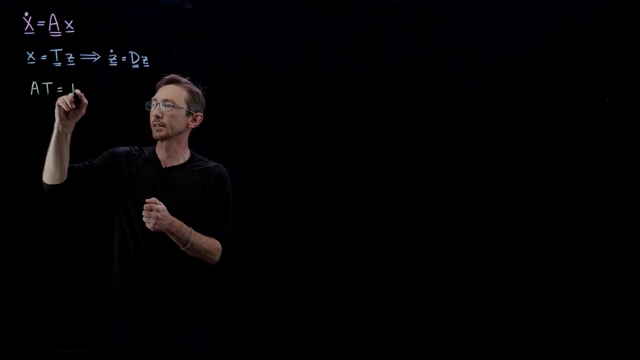 where a is not diagonal And, specifically, we derived the eigenvalue eigenvector equation for the t's and the d's where this is possible. Specifically, a times t equals t times d. This is the eigenvalue problem. Columns of t are eigenvectors of a, The diagonal elements of d. 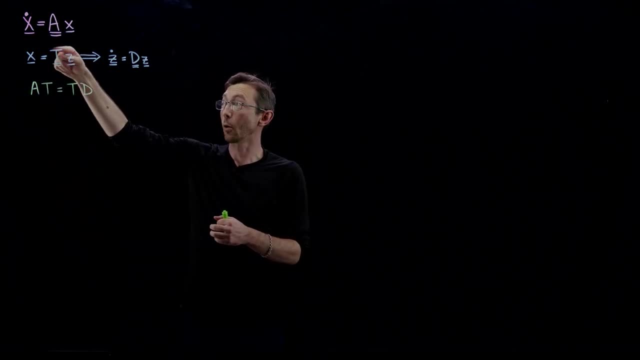 are eigenvalues of a, So the coordinate transformation is going to be a little bit different. So the coordinate transformation that diagonalizes a are specifically the matrix of eigenvectors of a And the d, the diagonal system that you get after doing that, these diagonal entries. 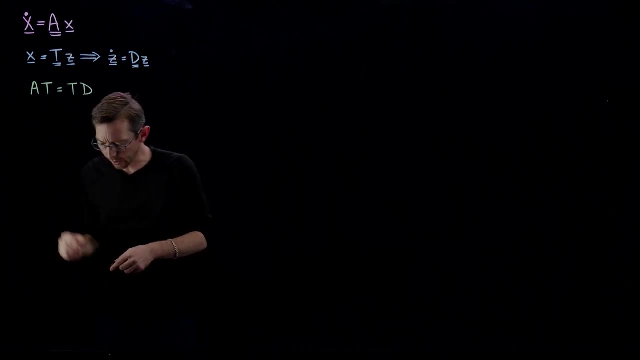 of d are the eigenvalues of a Good. So I think I want to just show a couple of things. I'm going to do a little bit of Python MATLAB demonstration here, just to convince you that yes, in fact d equals. what did I have? 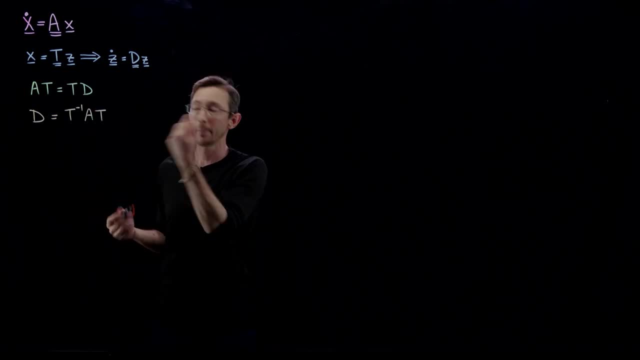 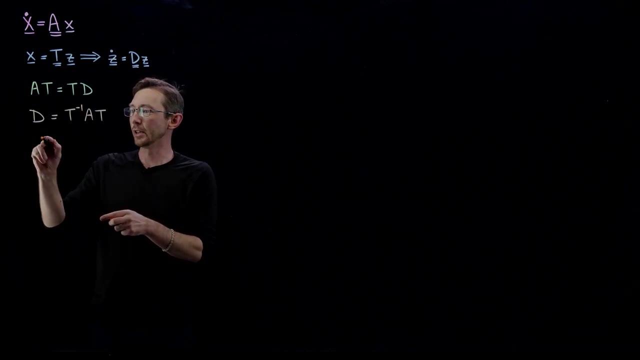 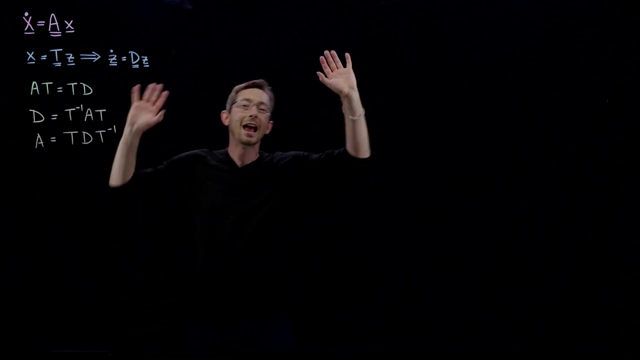 T inverse a. t is true. And also, conversely, that if I had d and t, that a would equal t times d times t inverse. Okay, And it's really really, really easy to compute eigenvalues and eigenvectors in MATLAB and Python. So I'm just going to show you that real quick. And then what? 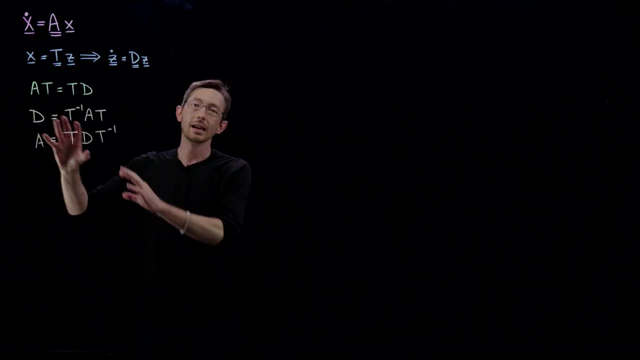 I'm going to do kind of the culmination of this set of lectures is I'm going to use- I'm going to assume that we've gotten a. we've decomposed a into its eigenvectors t and its eigenvalues d, So you know, however, means you know Python or MATLAB. we started with a and we. 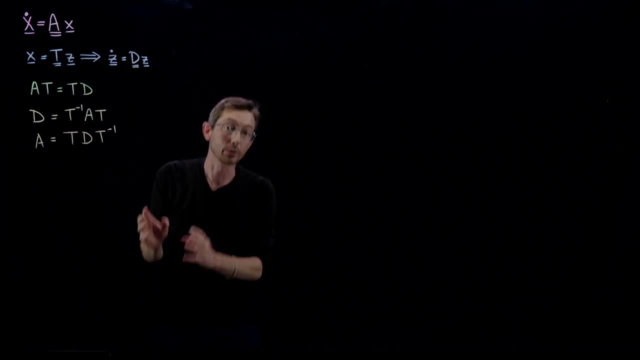 solved for t and d, And then I'm going to show you that with those matrices I can solve my original system of equations up here. So this is like my favorite lecture in differential equations so far, And so I'm just going to show you right now. 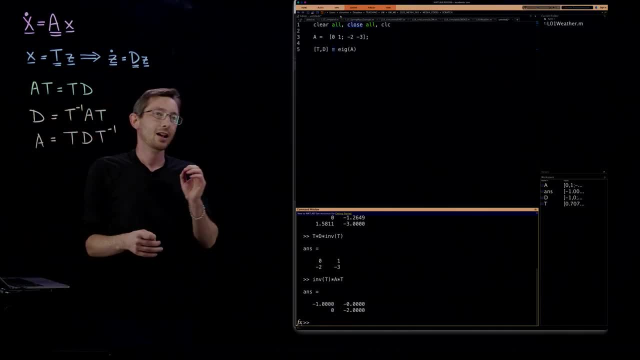 So the first thing I'm going to do is I'm literally just going to confirm, in fact, that you know it's easy to get eigenvalues and eigenvectors. I guess I'm going to start in MATLAB, So I'm 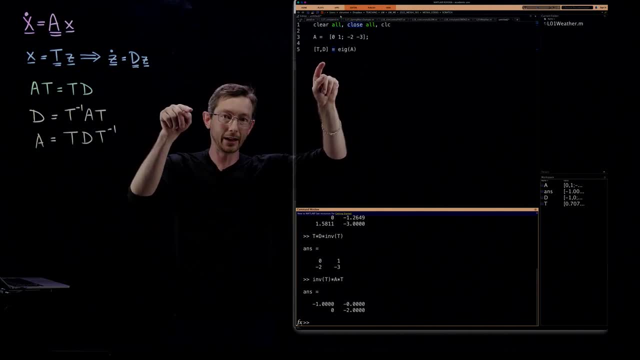 creating an A matrix: 0, 1, negative 2, negative 3.. And all I'm going to do is get its eigenvectors t and its eigenvalues d using the eig command, the built-in eig command. So it's literally one. 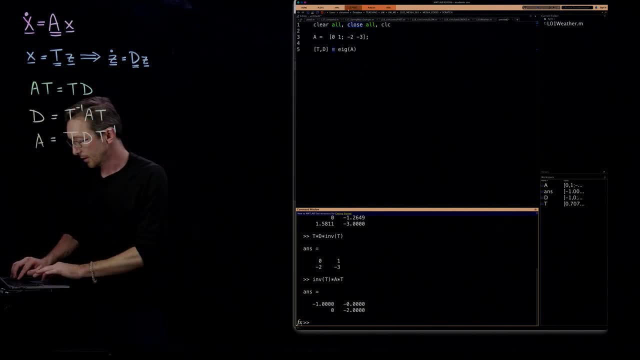 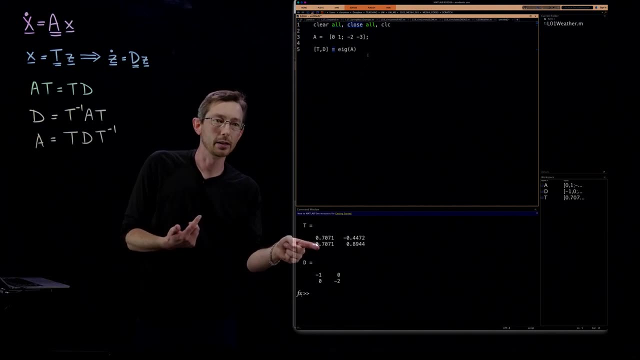 line to get all of the eigenvectors and all of the eigenvalues. So I'm just going to, you know, run that And so t our eigenvectors 1, okay, so it normalizes them so that they have. 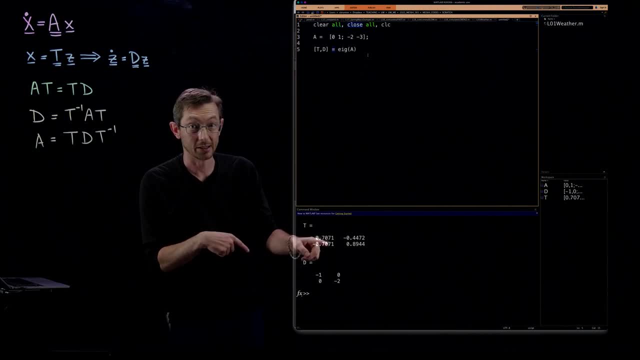 length 1.. So if you take, you know, this entry squared plus this entry squared, it'll have length 1.. Same with this, But essentially you can think of this as you know, the 1, negative 1 direction. 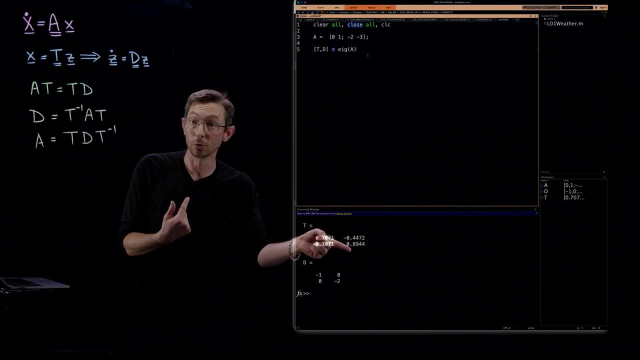 And this is the- I guess it looks like the minus 1, 2 direction And what I'm going to confirm for you. and then our eigenvalues are negative 1 and negative 2.. So I'm going to confirm these two expressions here. So, if I take 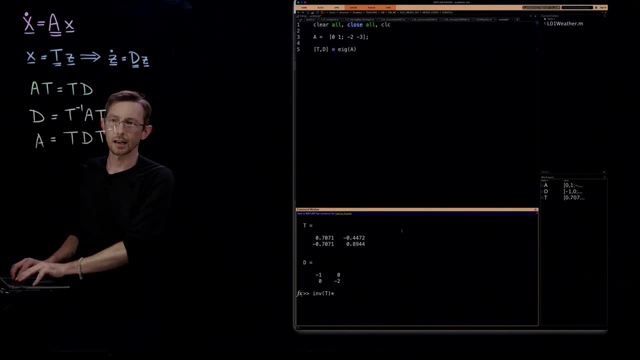 inv of t times a times t. that had better equal my diagonal matrix And yes, in fact it does Minus 1, 0, 0,, minus 2.. And I'll confirm the other one that, if I take. 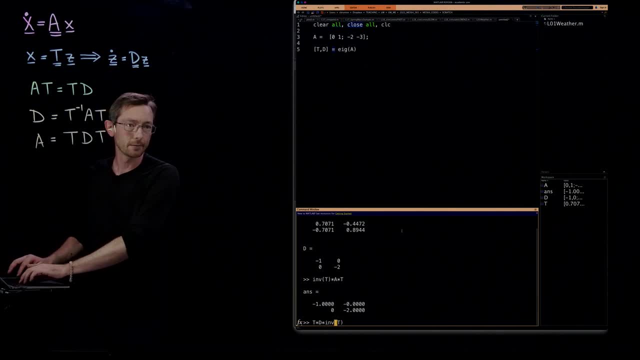 t times my diagonal matrix, times the inv of t, that should equal my original A matrix And in fact it equals 0, 1, minus 2. Minus 3.. Good, Quick sanity check. It's real easy to get eigenvalues and eigenvectors One line of. 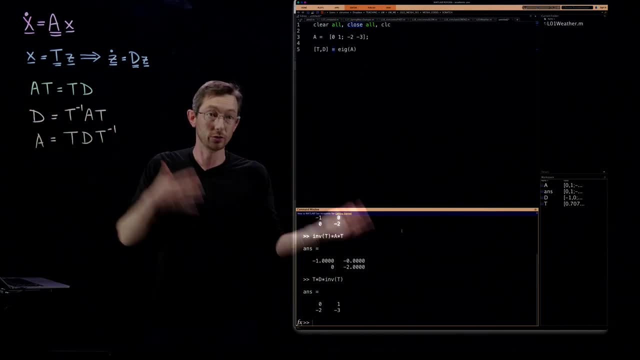 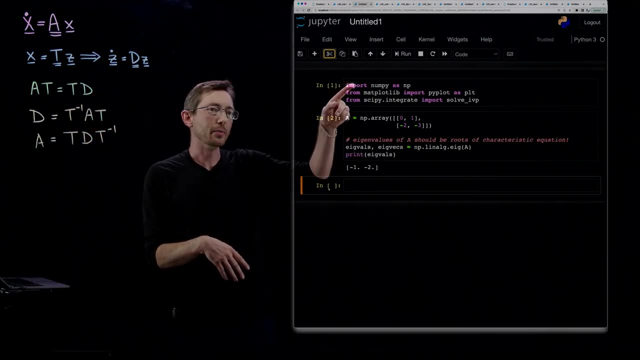 MATLAB And these properties that we think should hold do in fact hold. Let's just do kind of similar things in Python. Here again, you can. you know, import numpy as np. I actually don't need these other ones. This is just from another script. So I'm going to create an array, the same array. 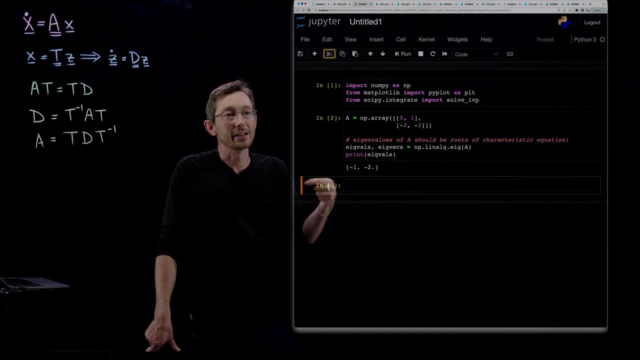 0,, 1, minus 2, minus 3.. And it's just as easy. So you get eigenvalues and eigenvectors. It's just, you know, from np lin alg, It's again the eig command, So just eig of a, And it spits out eigenvalues and eigenvectors in these. 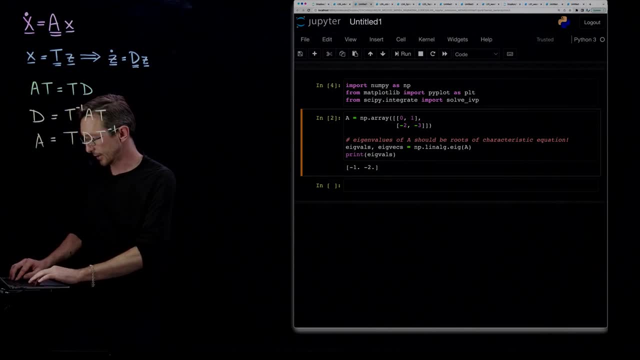 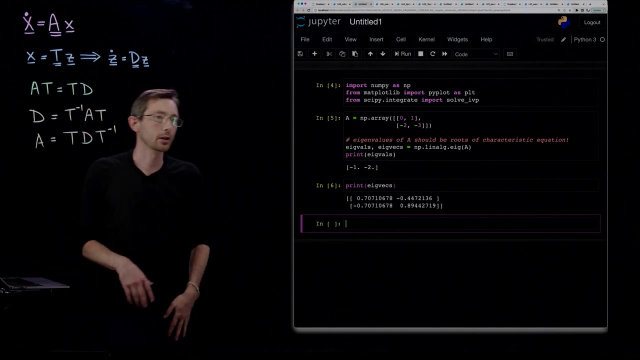 structures. So I'll just run this Run run And it printed out the eigenvalues If I want to. what's happening? If I want to print the eig vex, that should also work. And again, it is normalizing them to be unit, unit norm. So you can define your eigenvector, Any vector along an. 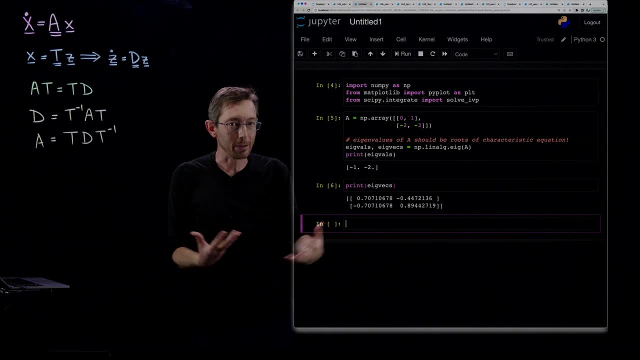 eigenvector- direction is technically an eigenvector. We usually pick the convention that our eigenvector has a unit length That uniquely determines it. Okay, And these are the same as before, And so clearly these are also going to hold. Good, That's all I wanted to show you in. 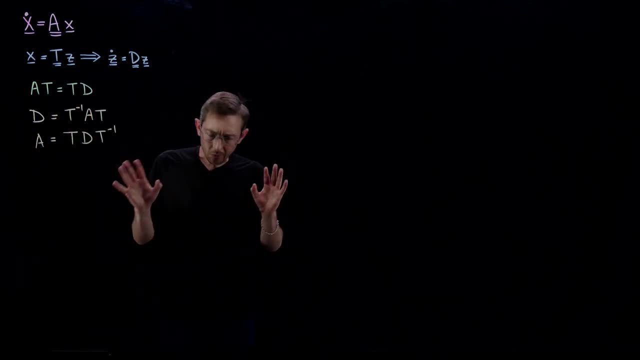 code. So now what I'm going to do is: we are going to, we're going to, we're going to, we're going to use these diagonal matrix D and these eigenvectors T to solve our differential equation. Okay, And so we know that it's quite easy to compute. It's easy to compute the solution of this, This: 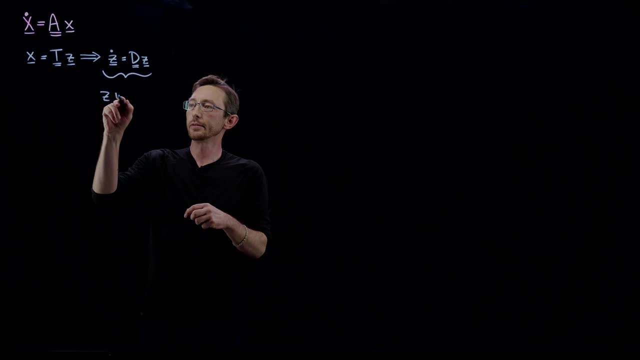 is just Z of T equals E to the matrix D time times. whatever initial conditions I have, I should probably write that down. I should probably write that down. I should probably write that down. My initial conditions I have, you know, X at time zero are my initial conditions And those initial. 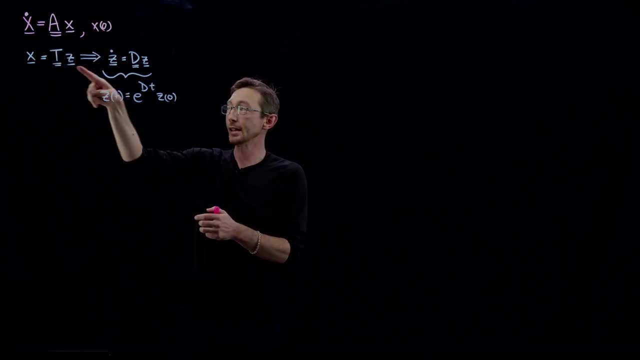 conditions are going to, you know, have a corresponding initial condition in Z. This is literally Z naught is T inverse X naught. That's pretty simple, And I'm you know we're used to thinking that the solutions of differential equations X dot equals lambda X. If I had 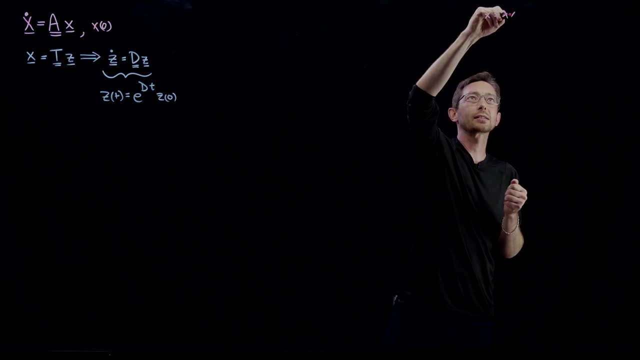 um, if I had X dot equals lambda X for a scalar X and for a lambda uh and I had some initial condition, then the solution would be: uh, X at time. T equals E to the lambda T times my initial condition: E to the lambda T times X naught. 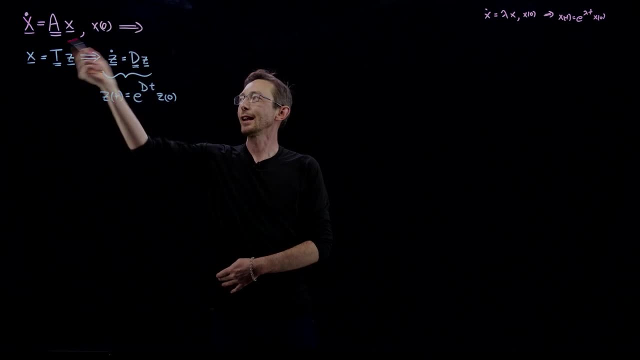 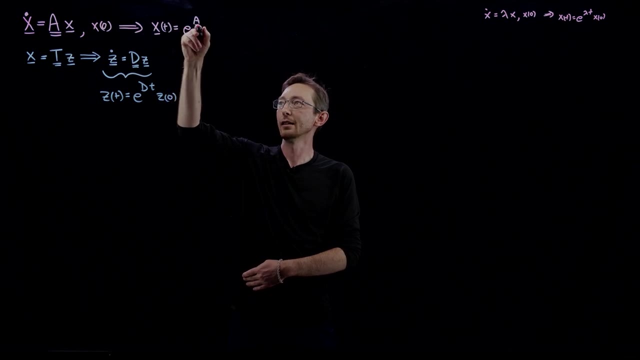 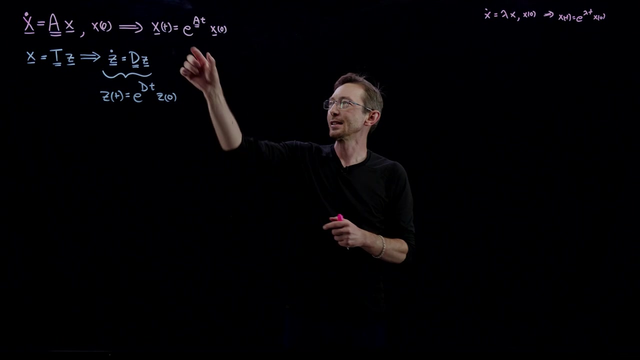 And so here I'm guessing that I get something similar, that X, my vector X at time T, is probably going to be E to the matrix A times time times, a vector of initial conditions. Okay, Now the question is: how do I compute this matrix exponential? I haven't shown you how to do. 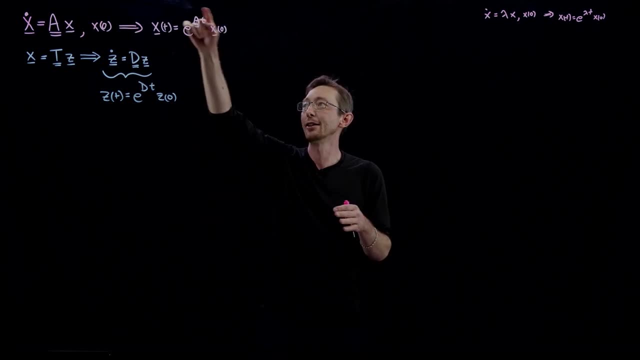 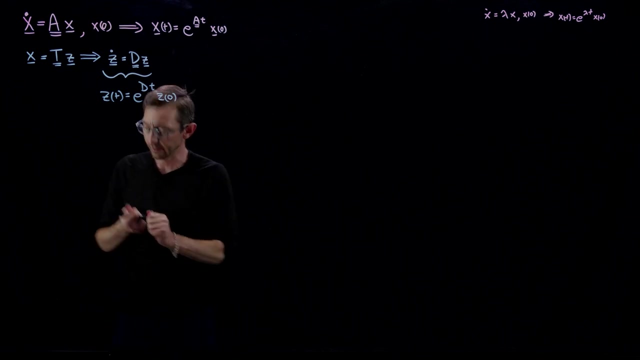 this, Um, so that's kind of one of the things I'm going to show you in this lecture- is how do you compute this matrix exponential and how do you use T and D to make it really easy to compute this thing. Okay, Um, so I shouldn't have erased all of my stuff. So we know that A is equal to um. 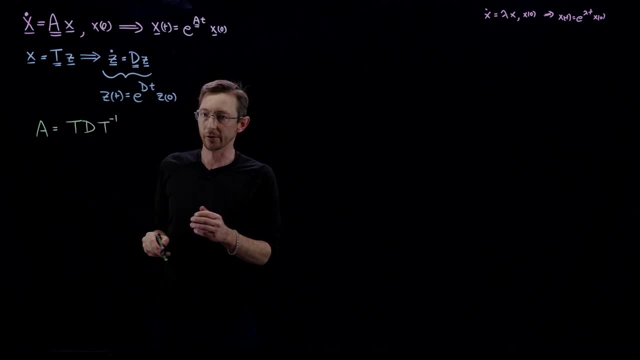 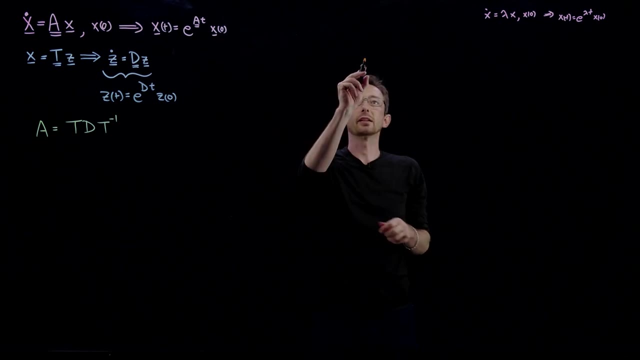 T, D, T inverse. What do I want to do here? I want to tell you that this matrix exponential- sorry, I'm skipping a step here- This matrix exponential E to the A, T- and I'm going to drop the underbars- We know that A is a matrix. I told you before that you can take the power series. 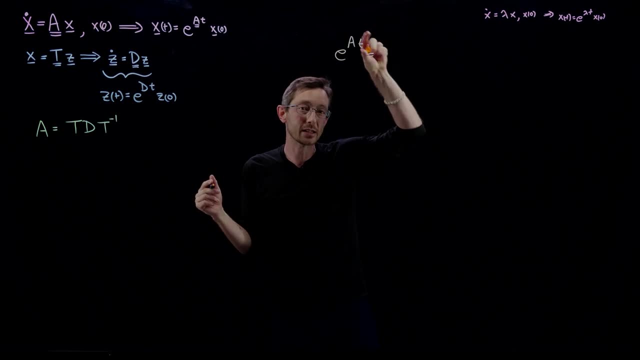 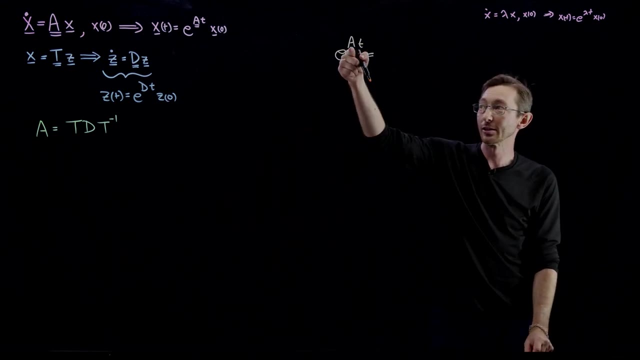 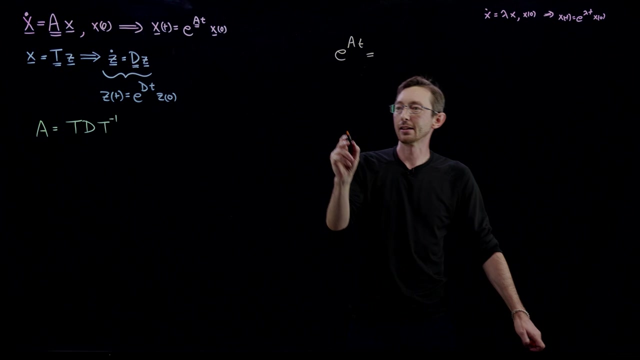 expansion for the exponential E to the X, and you can substitute in this matrix A, T every time you write that variable X. So the power series expansion of exponential says that this should be um. I'll write E to the X, So um E to the X is just one plus X plus X squared over two. 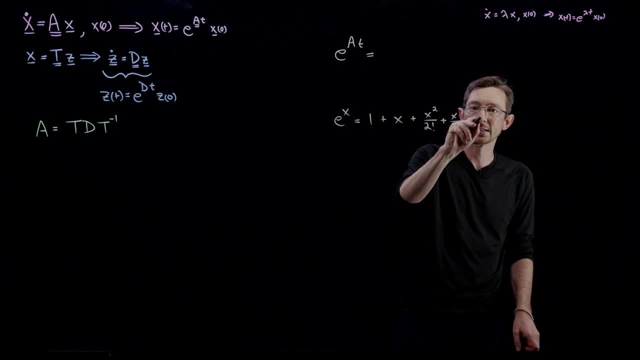 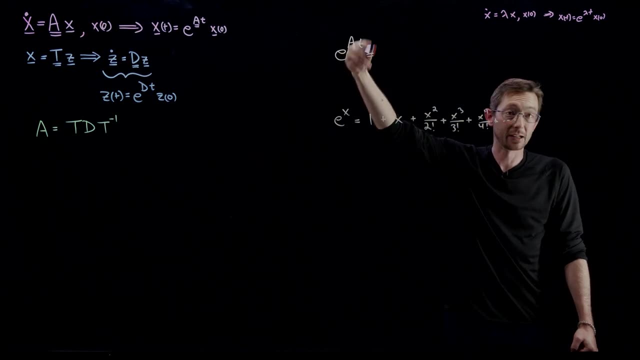 factorial plus X cubed over three. factorial plus X to the fourth over four. factorial plus dot, dot, dot, dot dot. And so this, this is going to be a matrix. This isn't going to be a scalar, So instead of one, it's going to be the ideal. So this is going to be the ideal, So this is going to be. 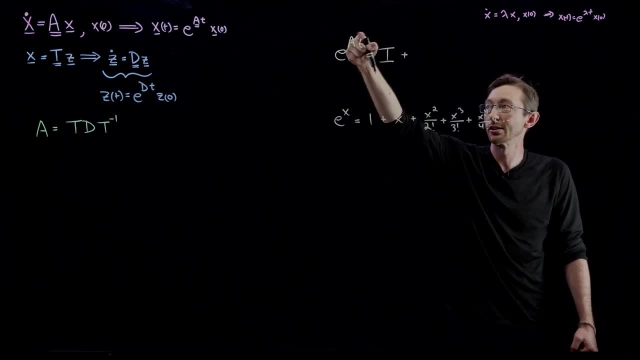 the identity And instead of X it's going to be, I'm going to substitute in A T every time I see an X. So, plus A T plus A squared T squared over two factorial plus A cubed T cubed over three factorial plus dot, dot, dot, dot dot, forever and ever and ever. Now computing these matrix. 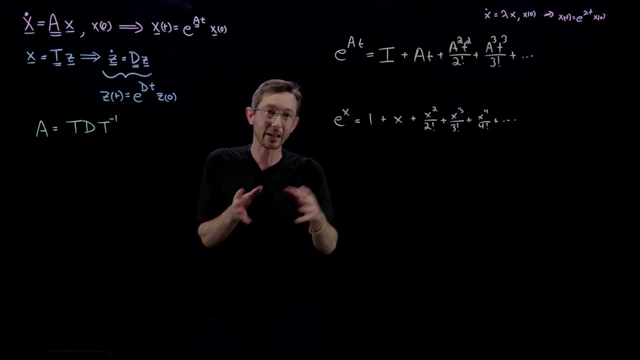 powers is going to get pretty tedious pretty fast, Like matrix multiplication is not cheap for big matrices, So I don't want to be actually computing all of these matrix powers And so I'm going to use T and D and special properties of those to make it really really easy to compute these things. 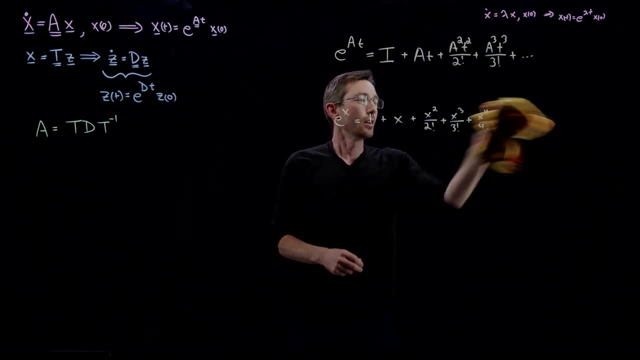 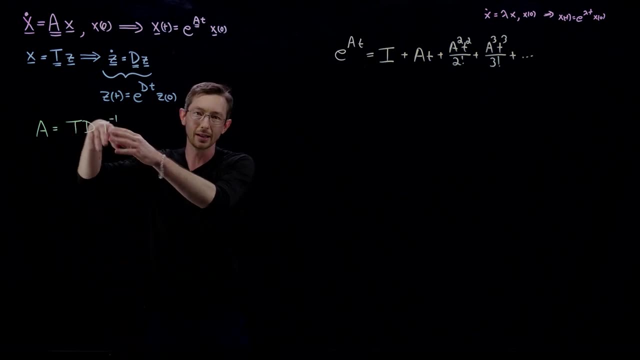 That's, that's kind of uh, what I'm going to show you now. Okay, So, um, we already know that A equals T, D, T inverse. That's fine. We computed this using, you know, the IG command and Python. 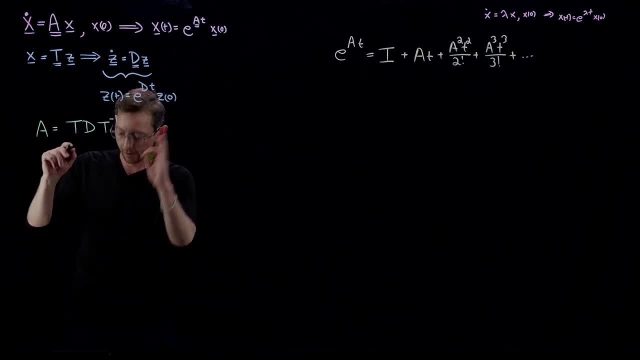 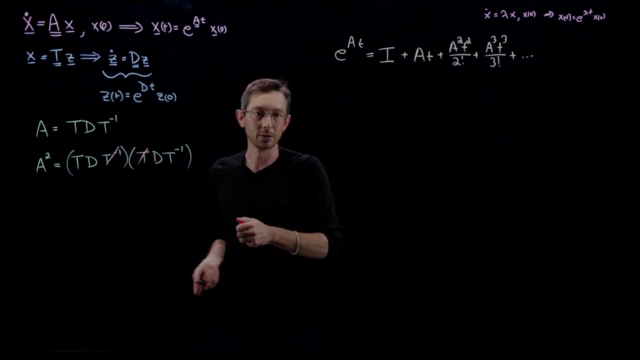 or MATLAB, And now I can write the A squared. This is where it gets pretty fun, So I'm going to write: the A squared is just this thing: times itself. So it's T, D, T, inverse times, T, D, T, inverse. But notice that I have a T, inverse times T, So these actually cancel out and this equals. 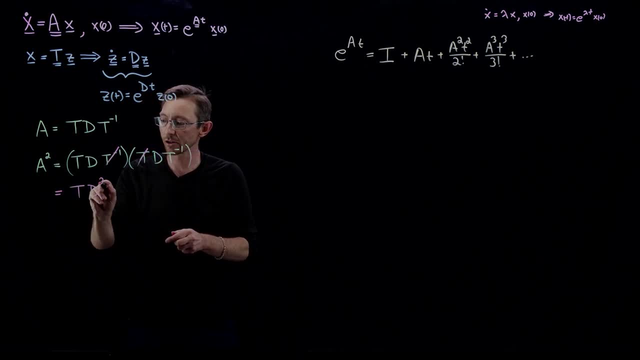 T times my diagonal matrix squared times T inverse. And this is actually not so bad. to compute D squared, D squared is easy. I just square all of the diagonal entries right Like a diagonal matrix times itself. A diagonal matrix squared is just the square of the diagonal entries. Okay, It's another diagonal. 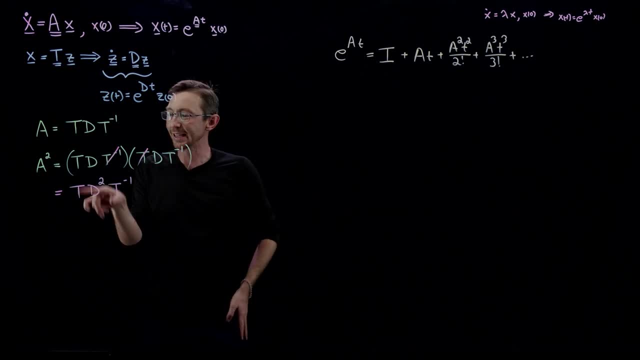 matrix where the entries are squared, So this is actually easier to compute. Similarly, we can compute uh A three A cubed, That is, uh T D T inverse times, T D T inverse. So this is actually gonna give us a. 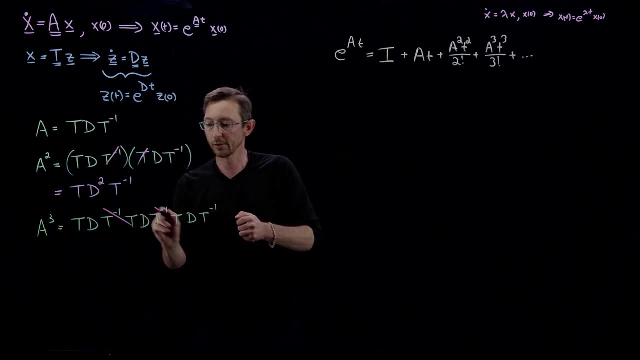 very pretty straightA predict or sentido. So so, t inverse times, T. I hope you're seeing the pattern here. T inverse Again. all of these in the middle cancel and I'm left with T. D to the third power. T inverse- again. this is really easy to compute: D cubed. that's just a diagonal matrix with all of. 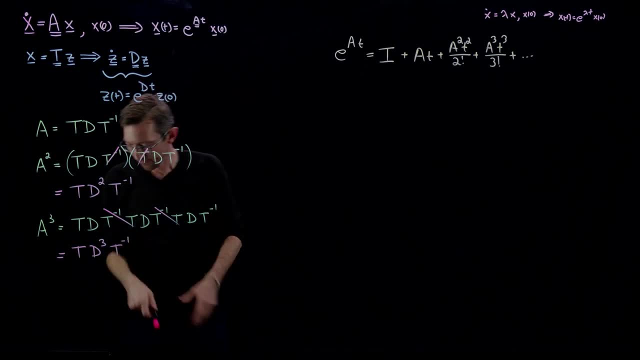 the entries of D cubed. That's nice And I can do this, uh kind of addудьH記 feature hé. So that's nice And I can do this kind of add guit mutation tremendous if I wantedNauseum if I wanted. dot, dot dot. That's just a diagonal matrix with all of the entries of D cubed, So that's nice And I can do this kind of ad. nee mouths음 plain hate. It should be an keerian. filter them if they want. It is�find Ahmedughiusm. it is written by memnatus troops, ahmed DE. 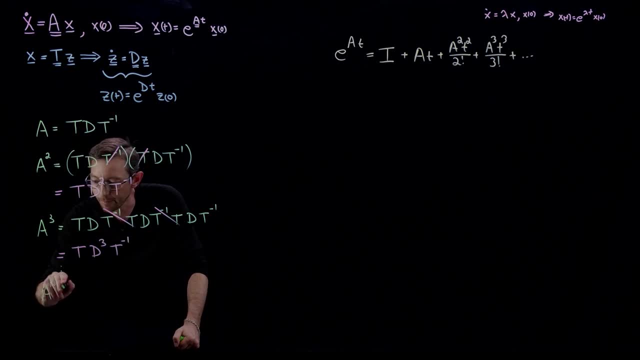 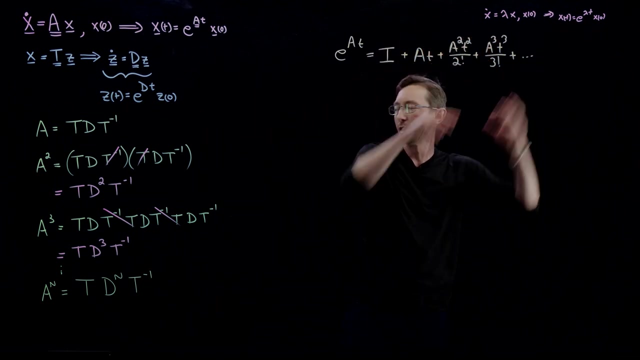 dot, dot a to the power n. the nth power of a is just going to be the same exact thing. It's going to be t, d to the power n times t inverse, And so basically every single term in here, whenever I see an a or an, a squared or an. 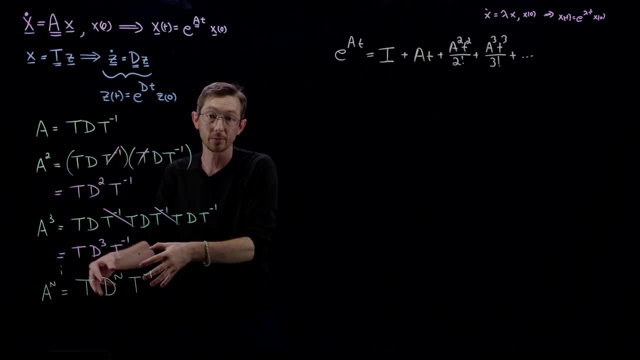 a cubed or so on and so forth. I can plug in these expressions in terms of its eigen decomposition, in terms of its eigenvectors and eigenvalues. Sometimes I call that its eigendecomposition. This is the eigendecomposition of a. 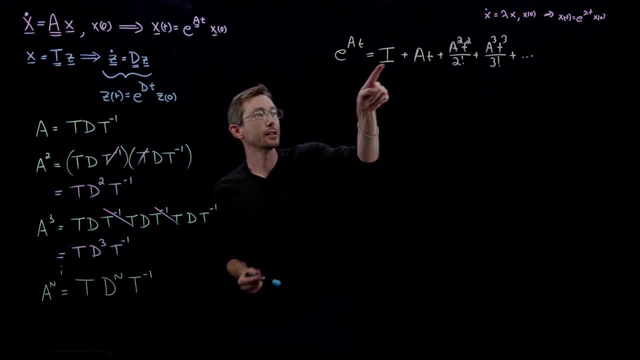 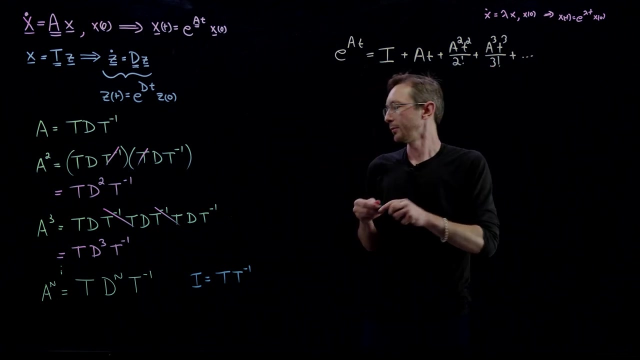 And I'm going to use one more fact, which is that this identity i can be written as t times t inverse. Okay, that's all we need to write this down. So what I'm going to write is that this expression here equals. maybe I'll use pink, since most 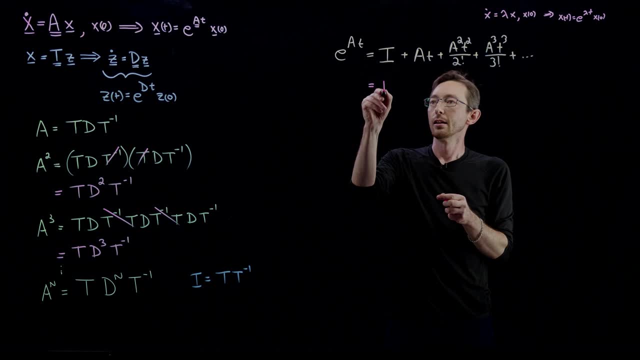 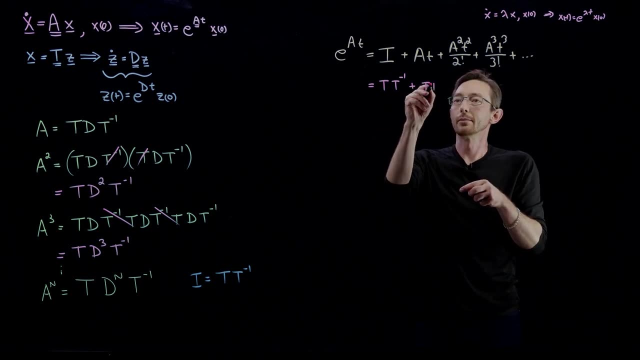 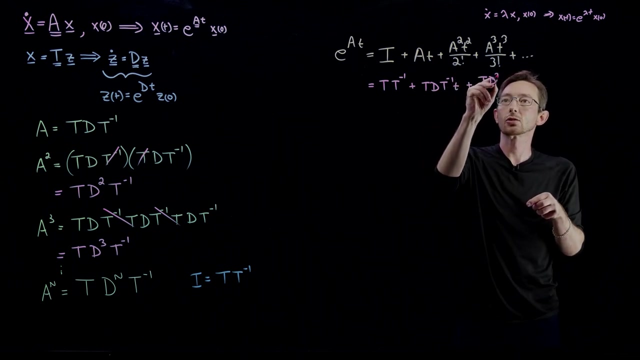 of these here are pink. So this equals t times t inverse Plus Plus t times d times t inverse: little time Plus t times d squared times t inverse: little time squared over two factorial Plus t times d cubed t inverse: little time cubed over three factorial. 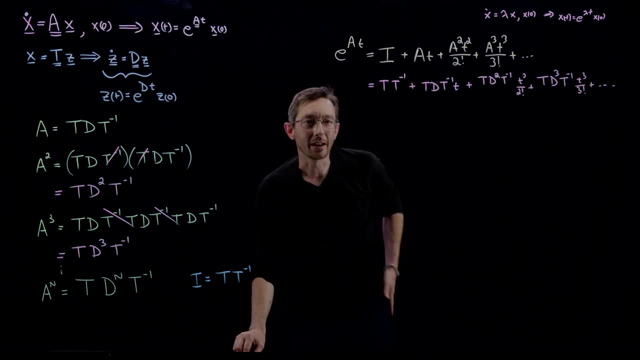 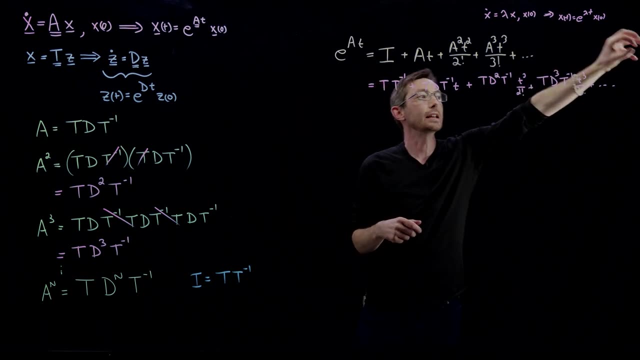 Plus, dot, dot, dot, dot dot, forever and ever and ever. And now what I can do is I can say that every single term in this has a big t on the left and a big t inverse on the right. 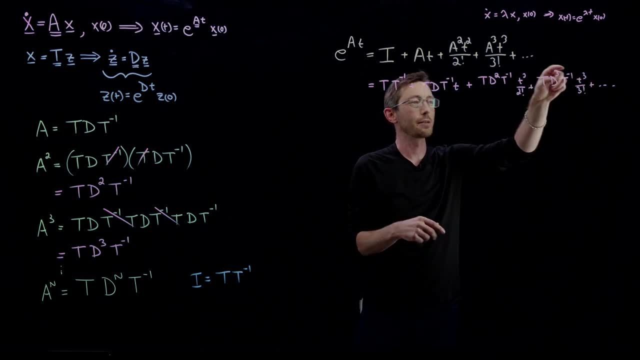 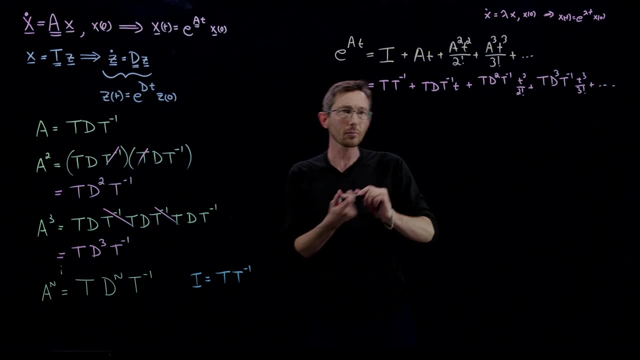 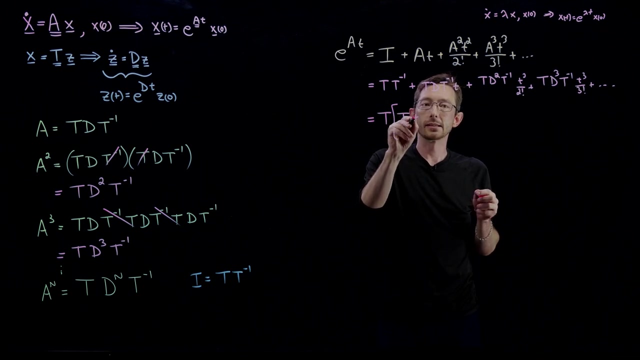 This scalar thing. I can move that anywhere because it's just a scalar. So the matrix part of this has a big t on the left and a t inverse on the right for every single term in this expansion, And so that equals big t times identity plus dot, dot, dot, dot, dot. a bunch of stuff. 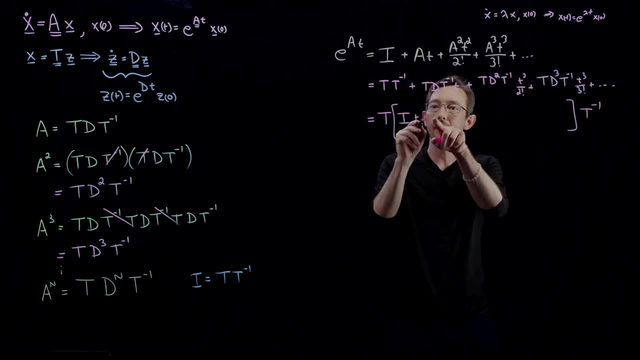 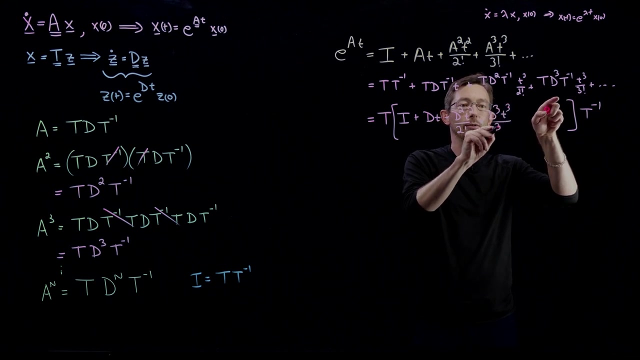 times t inverse. And this is the stuff inside is the identity- Plus a diagonal matrix t plus a diagonal matrix squared- t squared over two. factorial plus a diagonal matrix cubed- t cubed over three. factorial plus dot, dot, dot, dot dot. 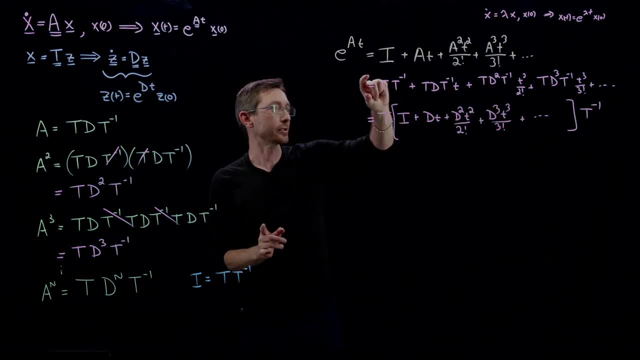 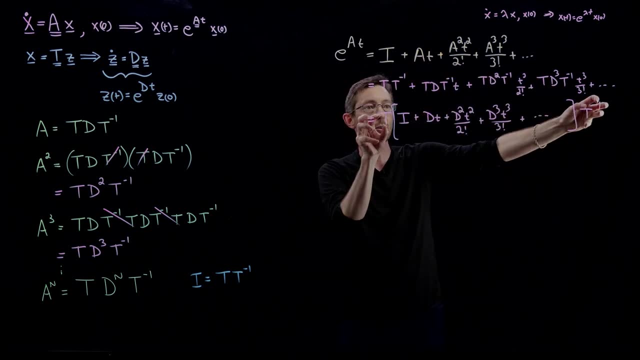 And now you'll see. so, like if that was too fast, just pause and convince yourself that this equals this. I literally just popped this big t on the left from all of these and this big t inverse on the right from all of these. 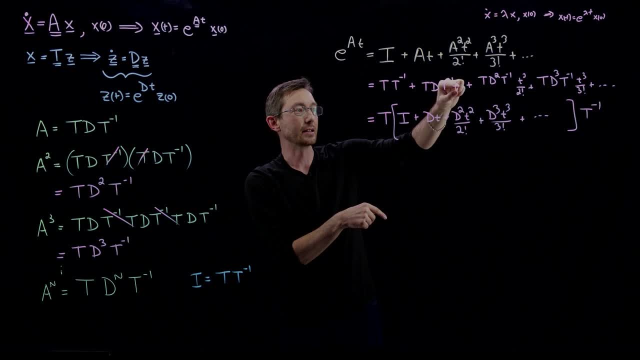 And then I collected all the stuff in the middle: Identity: Big d times t. big d squared, t squared over two factorial. d cubed, t cubed over three factorial. And now all of the stuff in the middle is actually really, really easy. 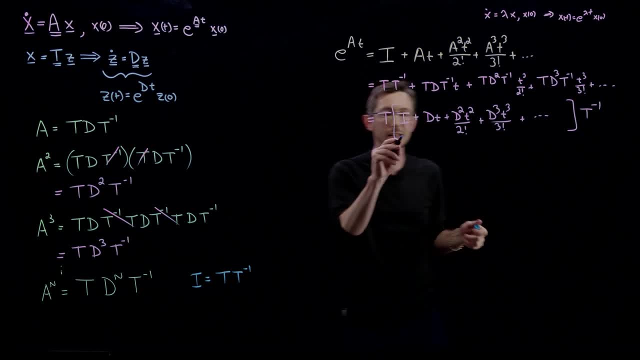 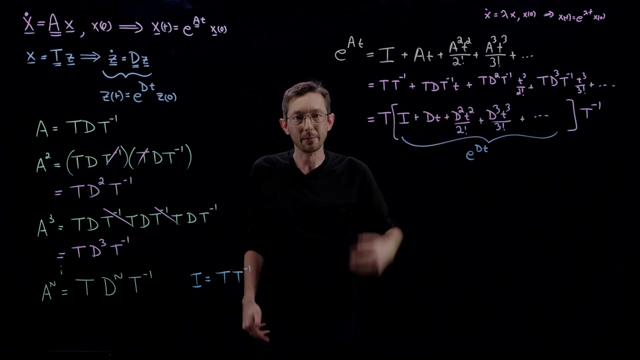 All of the stuff in the middle is the power series expansion, the representation of e to the diagonal matrix t. But we know that this is actually really easy to compute: All of these matrices, all of these powers of d are just still diagonal matrices. 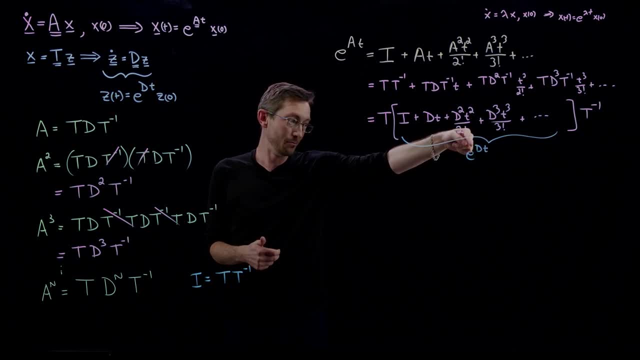 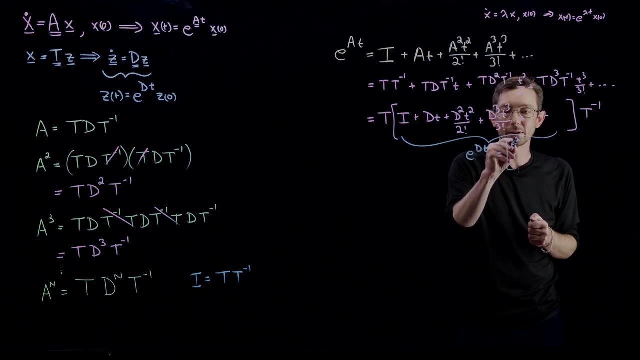 And so to get this e to the power matrix d times t, this is literally just a diagonal matrix. You know, e to the, e to the, With zeros everywhere else. I can just write this matrix exponential down for this diagonal matrix. 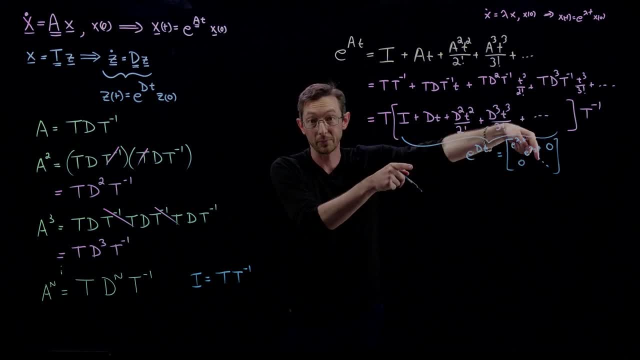 I don't even have to compute this, This is just I can write this down. Okay, so it's a diagonal matrix With to the lambda t's, And so now I hope you're seeing that, instead of computing this infinite set of, 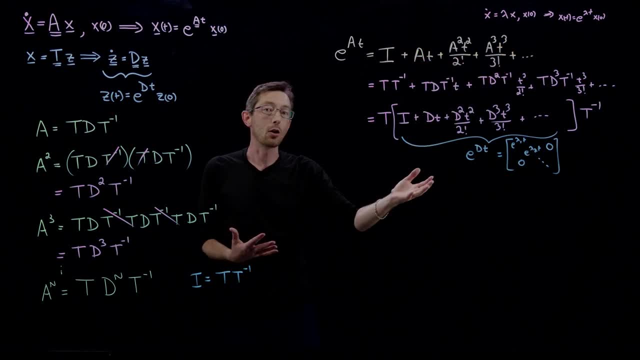 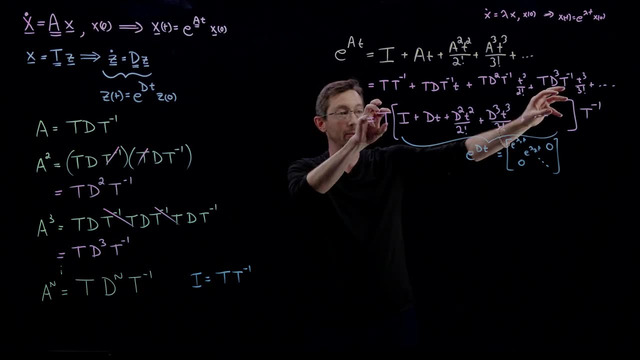 powers of a, which is going to be heinous to do now. all I have to do is compute the eigen decomposition. I get t and d. I compute e to the dt And I multiply it on the left with big T and on the right with big T, inverse. And that is my solution. My solution: x at time t, I'm going to. 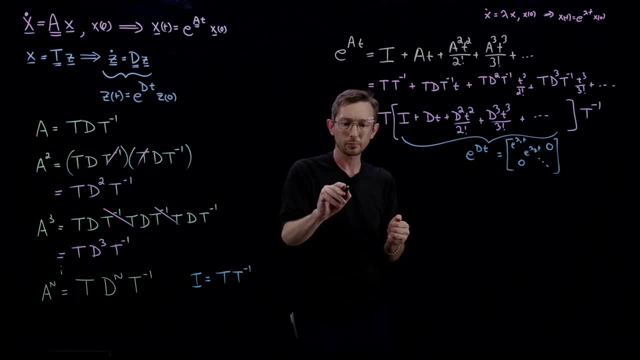 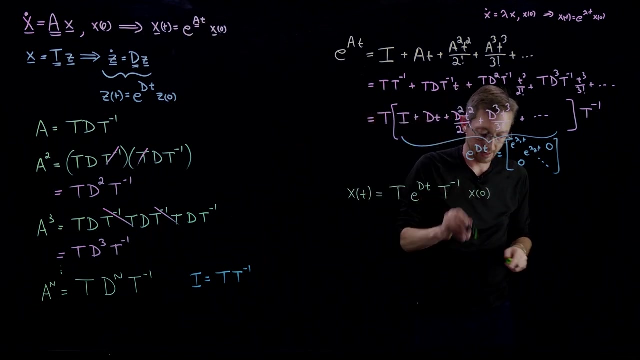 write this down. Maybe I'll write it down in green: x. at time t is equal to big T. e to the diagonal matrix times. time times big T inverse, That's e to the. at All of this is e to the. at times x naught. 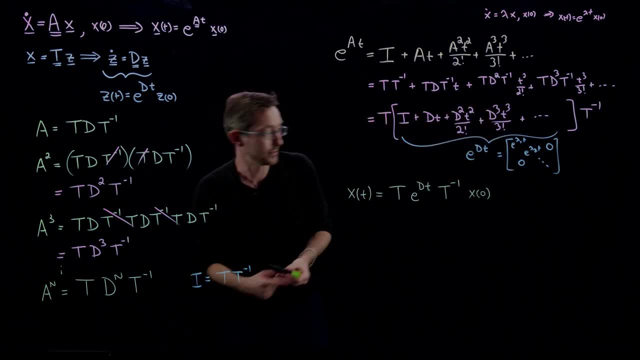 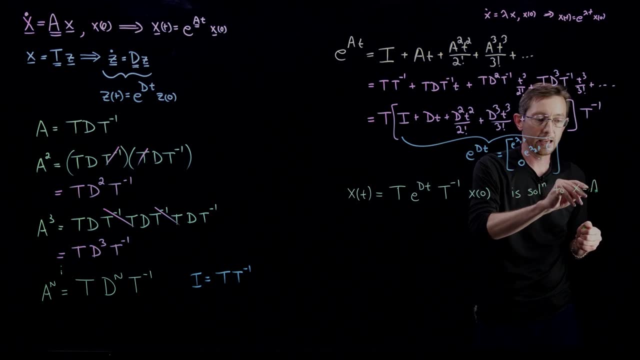 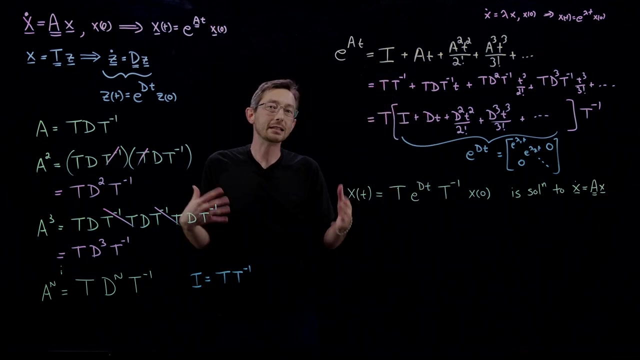 Okay, This is the solution. This is a. the solution to x dot equals a x, with this initial condition: x naught. Okay, So this is a big deal. We had this original differential equation that was really hard to solve. Maybe I could have guessed that this is. 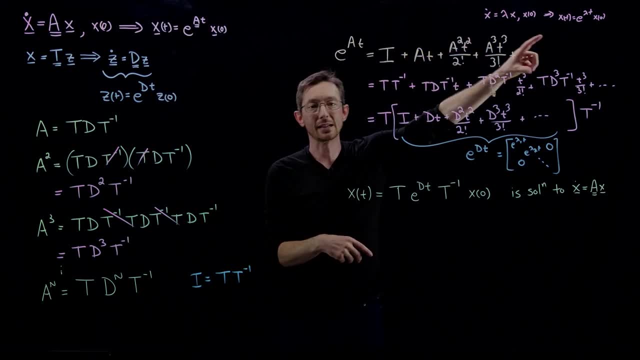 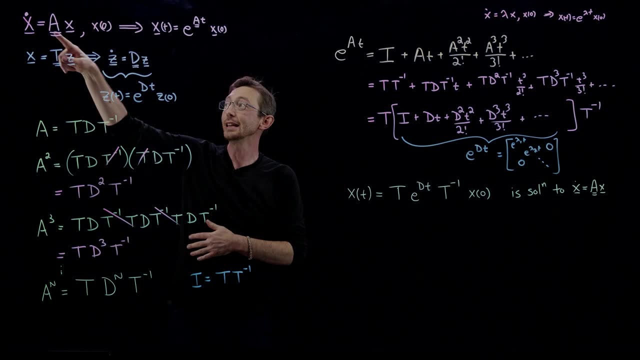 the form of the solution. But still, how do I compute this matrix exponential? This is going to be a nightmare to do for a generic, a matrix. So instead, what we do is we think, well, it would be a lot easier if this was diagonal. So let's find a coordinate transformation into: 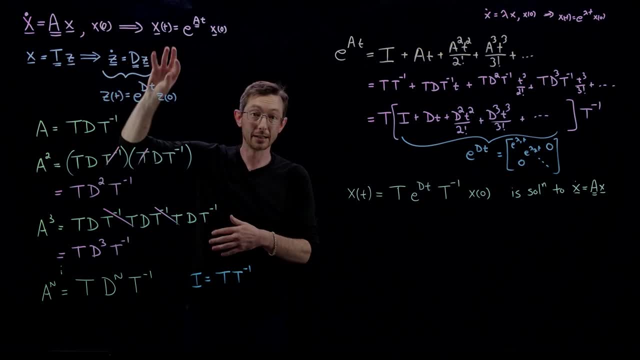 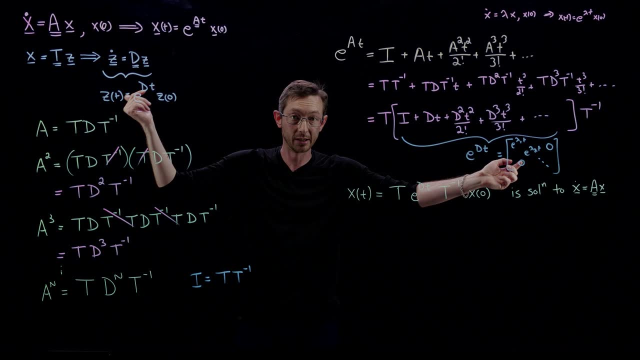 a coordinate system, z, where my dynamics are diagonal and decoupled. So I know how to solve that easily. It's easy to compute e to the diagonal matrix t. I do that by finding my eigenvalues and eigenvectors of this a matrix. So my eigenvectors t, my eigenvalues d, And then I. 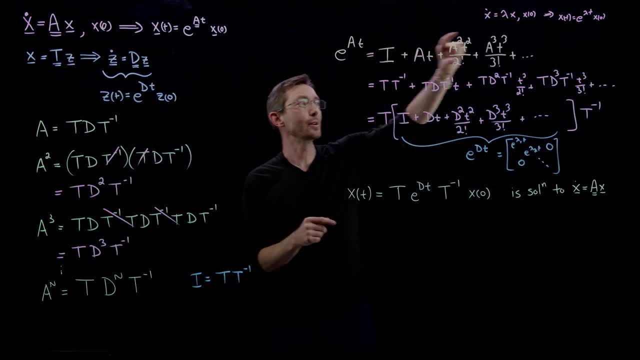 also find that those eigenvalues and eigenvectors make it much, much easier for me to compute this matrix exponential. I can kind of write: every time I see an, a matrix, I can write it in terms of its eigenvalues and eigenvectors. I can split terms and collect terms and get this very simple expression that that. 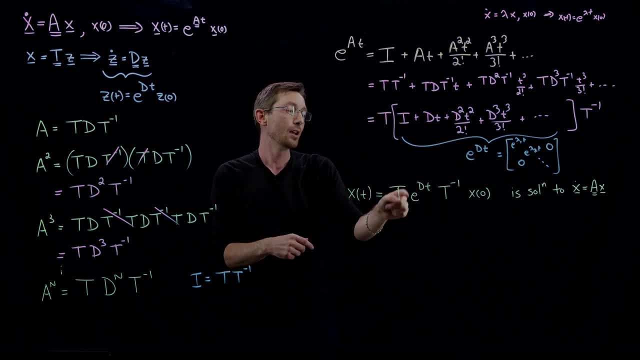 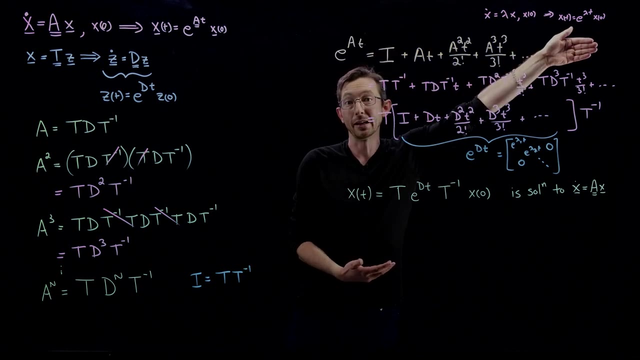 matrix exponential e to the matrix. a times time is a matrix. I know times a really easy diagonal exponential matrix. times another matrix. I know I can compute all three of these terms very, very easily, whereas I could not compute all of these infinitely many terms easily. 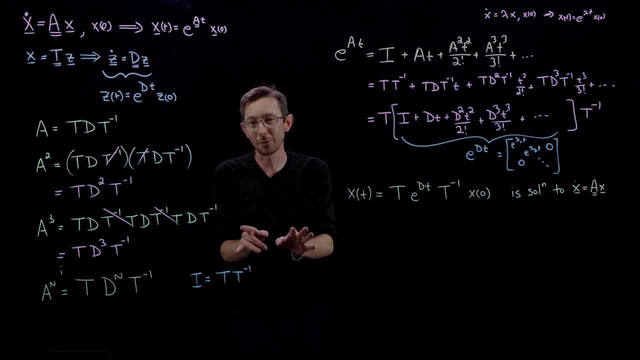 So this is much, much nicer, OK. one last thing I want to show you. This is kind of, for me, one of the highlights of this lecture is now. we're going to interpret this expression, this solution. So this is a big deal. This is the solution. We're going to interpret this step by step, OK, So this t. 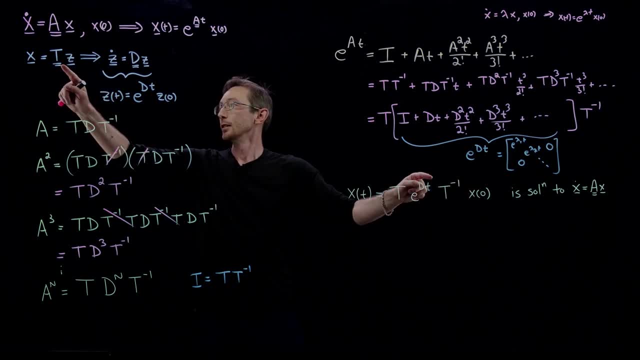 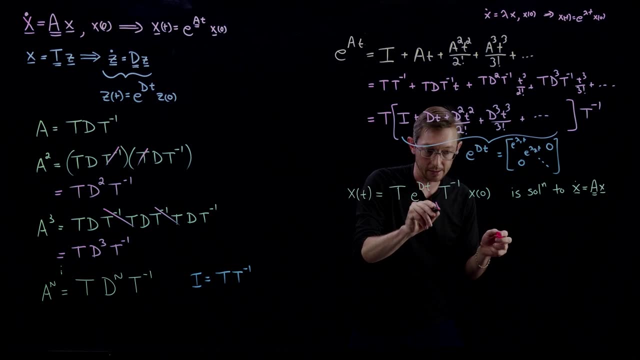 inverse times x naught. T inverse times x naught is literally z naught, So this term here this is, is Z naught. so essentially what we're doing is we are taking our initial conditions in the X coordinate system, in my original coordinate system that I, you. 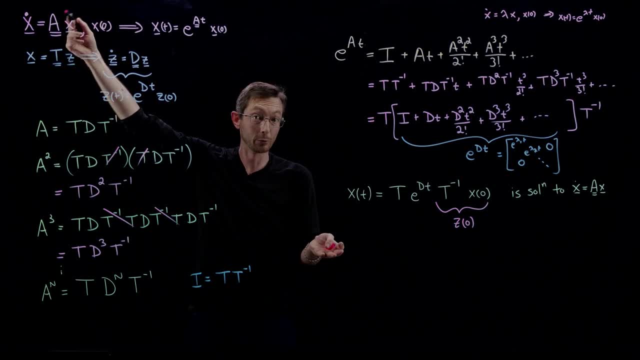 know I wrote down my dynamics in my original X coordinate system. for some reason. I must have had a good reason. so now what I'm going to do is I'm going to take my initial conditions, I'm going to map them through T inverse into a set of 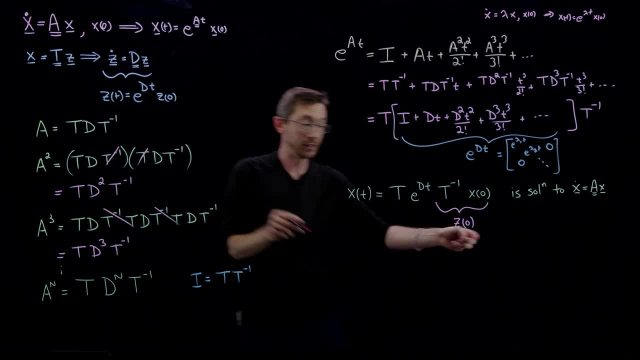 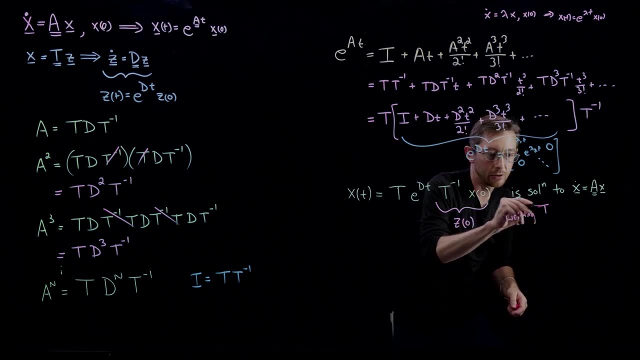 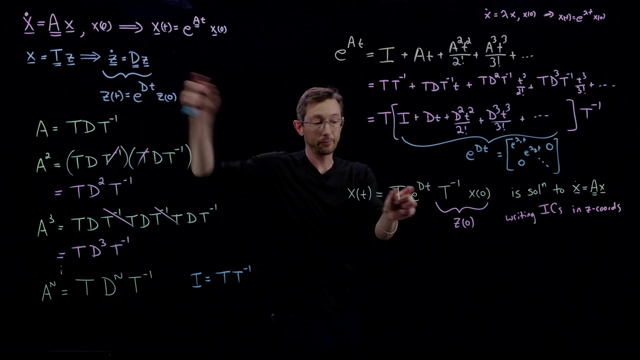 initial conditions in my nice Z coordinate system. so this is, you know, I'm writing, I'm writing my initial conditions in Z coordinates, in Z coordinates. then what I'm doing is I'm multiplying by e to the matrix D, T, so this whole thing: e to the matrix, the diagonal matrix D, times, time, times Z. 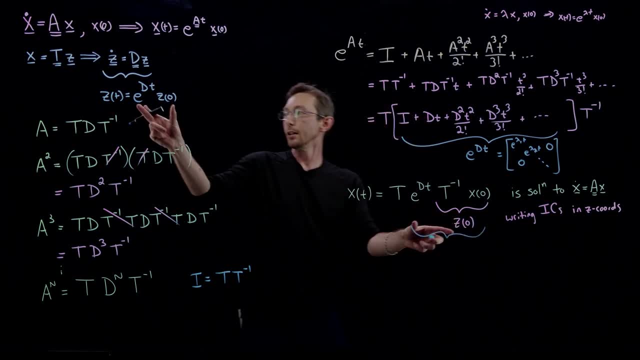 not, this is literally Z. at some future time. T, this is Z of T. so what I've done is I've taken my initial condition. I've mapped it into Z coordinates where it's easy to to write down the solution. it's easy to write down Z of T in these Z. 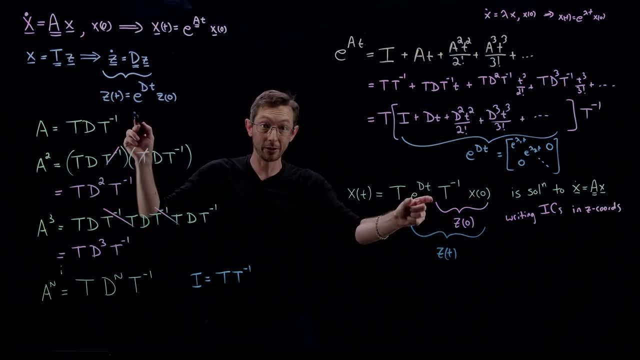 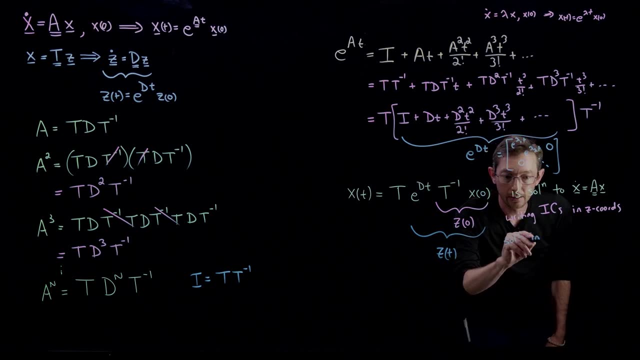 coordinates. it's just, you know my initial condition times this diagonal matrix, that's Z of T. so this is my solution in and Z coordinates, which is easy, and then, finally, what I do is: now I have the solution in Z coordinates, but again I wanted it in X. 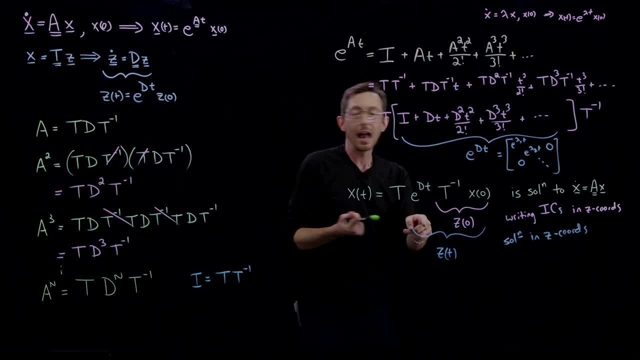 coordinates in the first place. I started in X coordinates and so to get back to X coordinates, I just multiply by a big T, that's multiply by a big T, and now I'm back in X. so now we're back to the solution in X coordinates and I think this is just really really cool, like this for me. 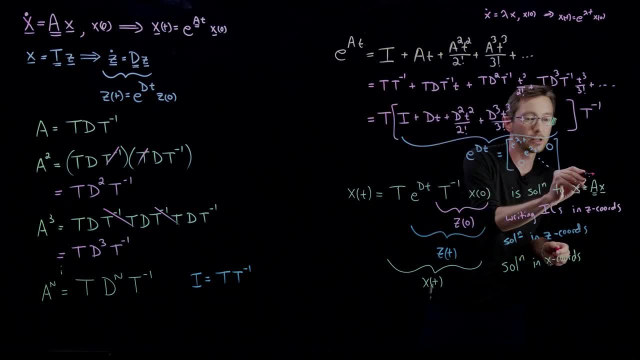 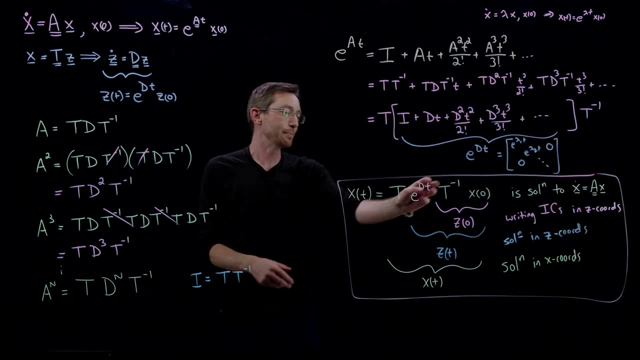 is one of my favorite pictures in differential equations- is this solution here and this real physical interpretation. these matrices T and D are not magic, okay, this is not eigenvalues and eigenvectors don't come out of nowhere. they are very, very simple and intuitive matrices that are useful for solving systems of differential equations. 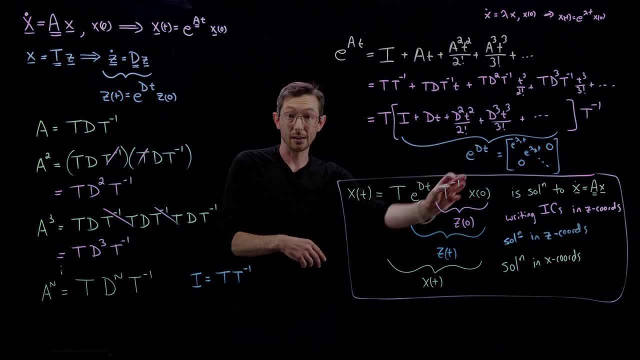 the T inverse matrix maps me from X coordinates into Z coordinates. my initial condition: X naught into Z naught in those Z coordinates. my dynamics are diagonal. this diagonal matrix are my eigenvalues of my A matrix and so it's easy to write E to the DT to solve. 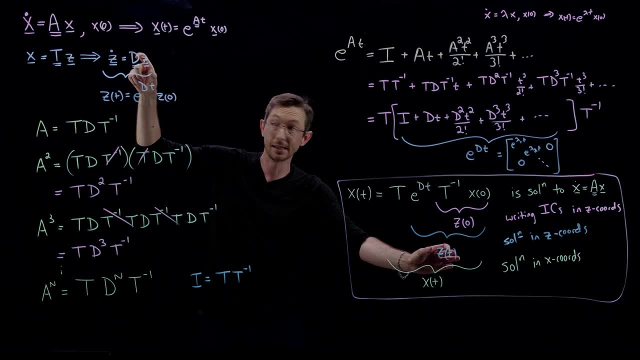 to move Z naught forward in time to Z at some future time and then to go back to my original coordinates. I'm going to go back to my original coordinates and I'm going to go back to my original coordinates. I just multiply by T again, so very, very intuitive. 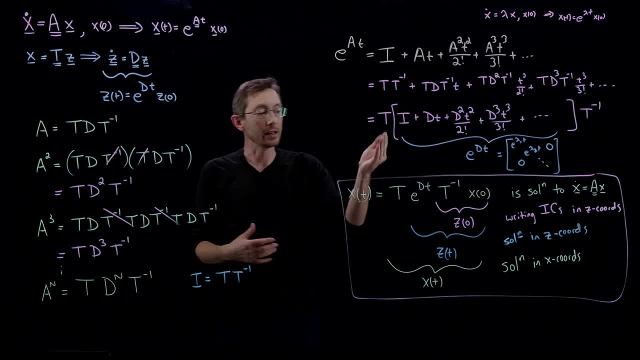 very, very kind of simple, in terms of eigenvectors and eigenvalues, how you solve X of T. okay, good, that was it. that was a big lecture. I'm ready to go home now. in the next lectures we're going to look at specific A matrices that have certain structure. 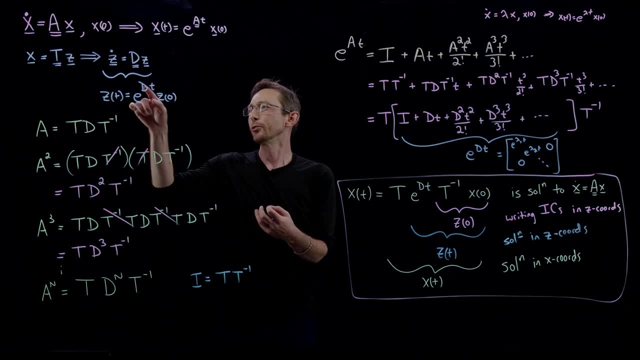 that have really interesting eigenvalues and eigenvectors. so, for example, when these eigenvectors are purely real and negative and negative, this will be a stable system. when they're purely real and positive, it'll be an unstable system. when they are imaginary, I'll have a rotating system. 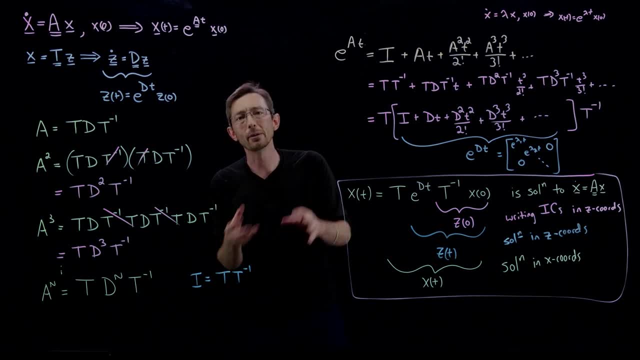 you know kind of oscillating system, cosines and sines, and I'm going to build up all of your intuition for these systems of differential equations, for the whole menagerie of the ordinary differential equations you can have in terms of these eigenvalues and eigenvectors. 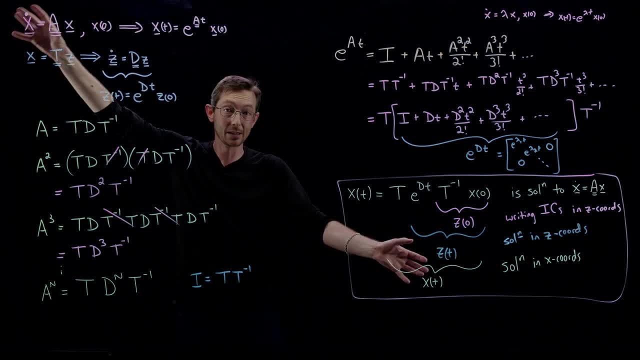 this is the new language we're going to use to understand these systems of equations. okay, that's all kind of it. thanks for coming up soon. thank you.